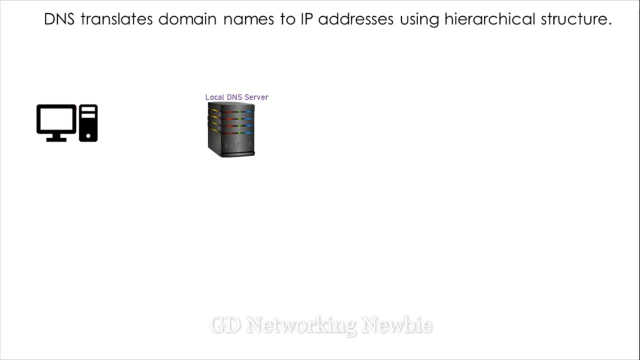 Hi everyone. So today we are going to discuss the hierarchical structure of DNS system. So DNS, a domain name system, actually translates the domain names to IP address And, as we discussed in our previous video, that all the computers, all the nodes are the electronic gadgets which are part of the Internet, has an IP address And if you want to get connected with them then we need an IP address. But that is difficult for the human being to do. 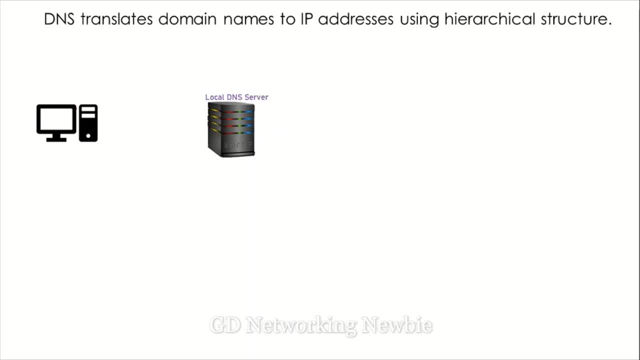 So we need to remember all these IP addresses. So we use names instead of IP address And DNS translates those names into IP address. So what happens when a user using any computer or any electronic gadget, if it types a URL by using any browser, then for that URL or for that domain we need to have an IP address. And to get an IP address that computer, the operating system within that computer, first checks its own memory to see if it already has an IP address. 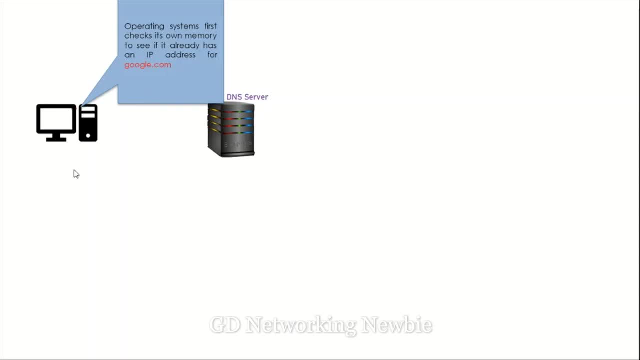 If it already has an IP address for googlecom, And if it finds, then it can can retrieve the contents from googlecom. But if this- this the cache memory- doesn't have an IP address for for googlecom, then what happens? this user sends a request to the local DNS server, And that local DNS server is normally provided by the ISP from where you get the Internet services- And in this local DNS server the request from the user. 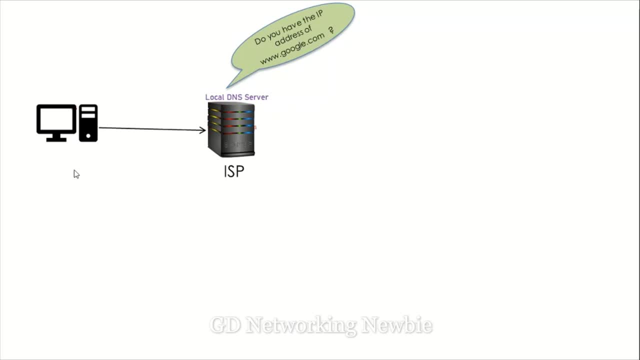 the user asks that: do you have the IP address of googlecom? And in response to that query the local DNS server has got an operating system and it first again checks its own cache memory to see if it already has an IP address. So first it checks its own cache memory to see if it has an IP address for googlecom And if it finds, then this, this: the local DNS server can forward that IP address to the local DNS server. 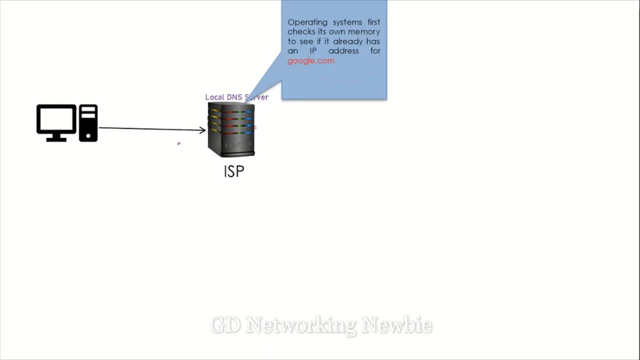 user back. So if it has, then it can send back the back the IP address to this user. But in case if this local DNS server doesn't have the IP address for the googlecom, then it will it will. it will request the root DNS server on behalf of the user to find out the IP address for googlecom And the root DNS server after receiving that request. 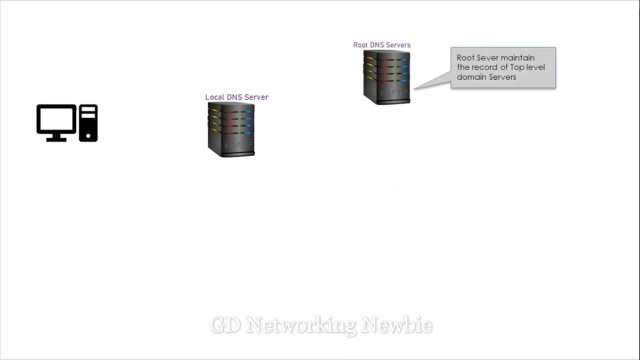 it will not have the actual answer or the actual IP address for the googlecom, But the root server actually maintains a record of top level domain servers, For example. for example, if we are looking for the IP address of googlecom, then this top level domain will have the, will have the record for these, this part of the domain name. So by looking at this top level of the URL, 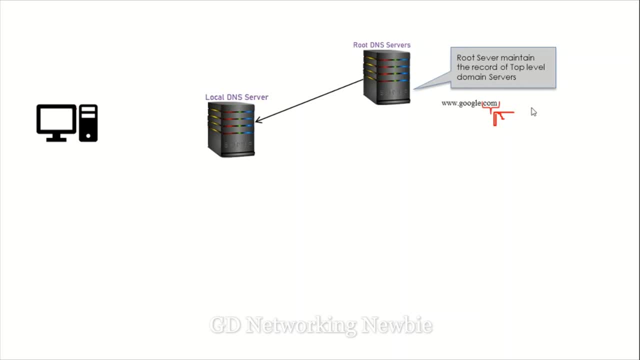 the domain name, the root DNS server will send an IP address of the top level domain server, which can have the IP address for googlecom and local DNS server. after receiving the IP address from the root DNS server, will forward the request to the top level domain server. 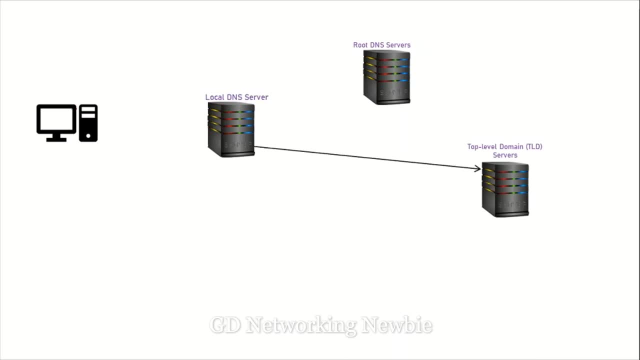 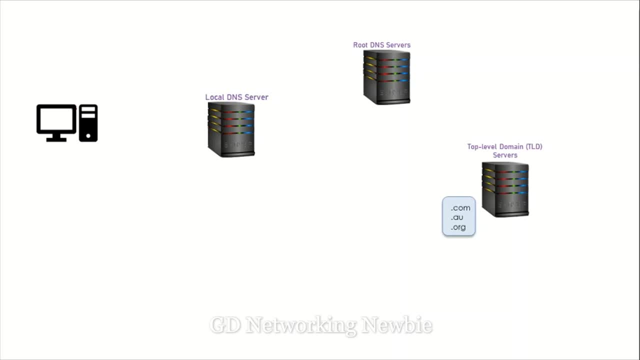 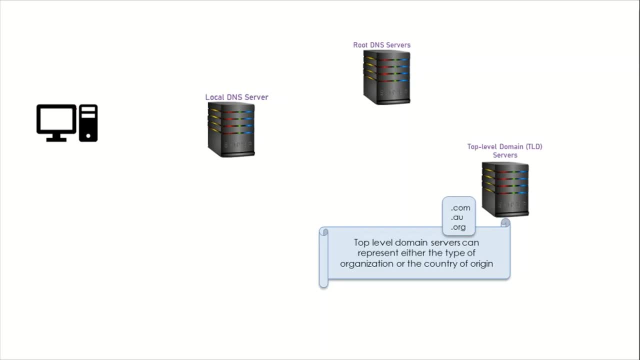 user back, user back of organization are the country of origin and this top level domain does not have the IP address for our domain name, but it has an address of the secondary level domain where we can find the IP address for the googlecom. so this will look at the second part. this will look at this part of the URL, or the. 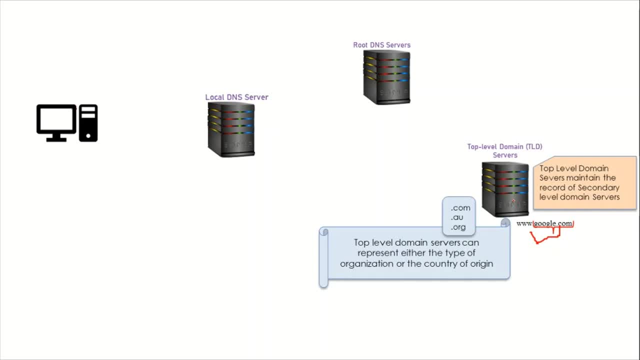 domain name and it will send the IP address for the next level of domains and servers. to find out, the IP address was there and this will send the IP address for the next level of domains to the local DNS server and the local DNS server. after receiving the IP address for the next level of domain servers, it 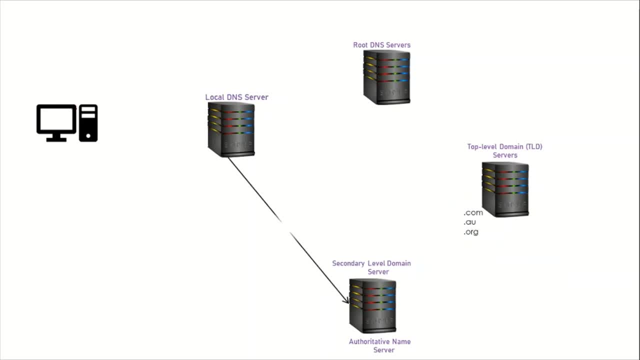 will send a request to the Secondary level domain servers to find out the IP address for googlecom. ok, so many times we saw this at the live sample. this is like the direct link, and now this secondary level domain server will have an IP address for googlecom. and then this: 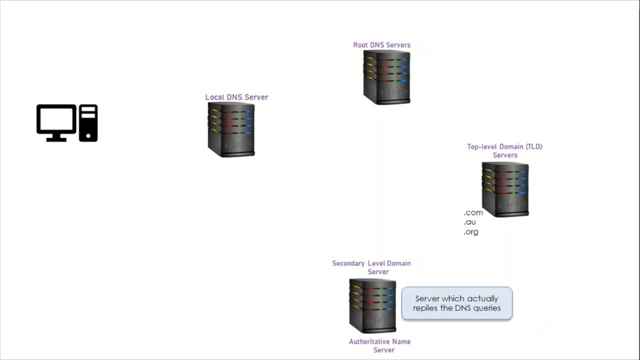 secondary level server actually resolves the IP address for the googlecom. so this secondary level, this specific secondary level domain server is also known as authoritative name server because it is going to provide- it is basically going to provide- the IP address for googlecom, so it sends an IP address to the local DNS server and the local DNS server after receiving. 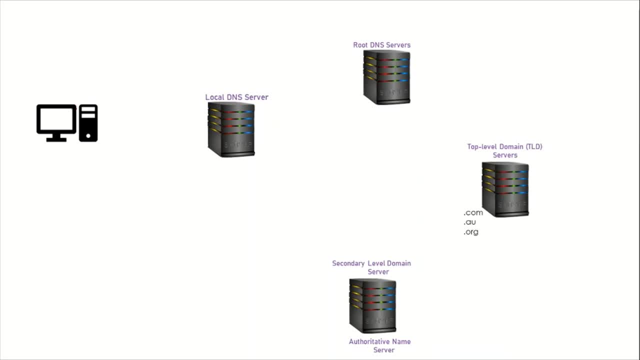 that IP address. it forwards that IP address to the, to the user, and that user, after receiving that IP address, can use that IP IP address to get connected with the domain of googlecom. so it uses the IP address and get it gets connected with the, with that domain and that. 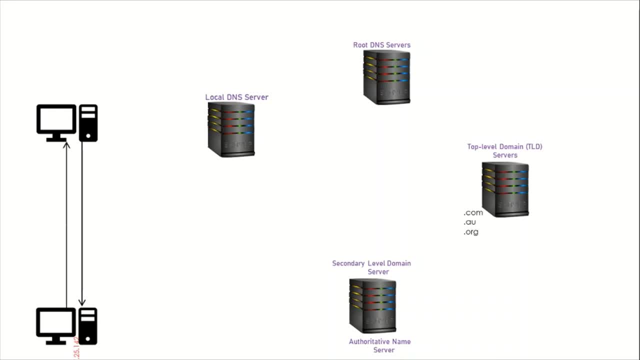 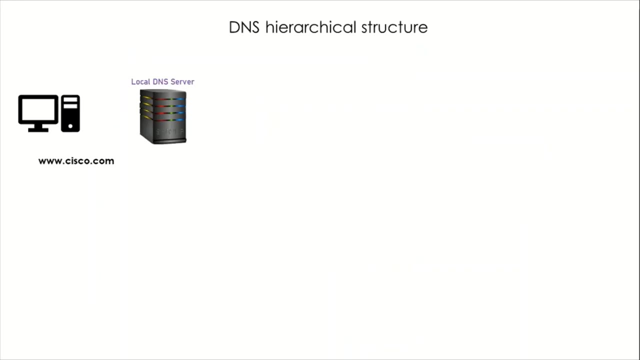 domain forwards back some data back to the user. and now how the user can display the web page requested by us. So this was the hierarchical structure used by the DNS system. Now, another way to look at the same is that in DNS hierarchical structure. 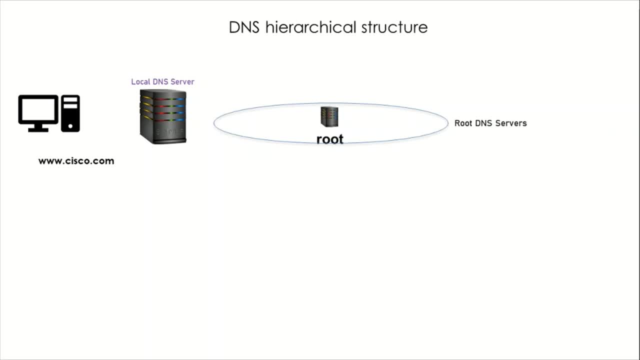 when a user types, for example, ciscocom, then what happens? first point of contact will be the root DNS server And the root DNS server will look at this part, at this part of the domain name And by looking at this part, 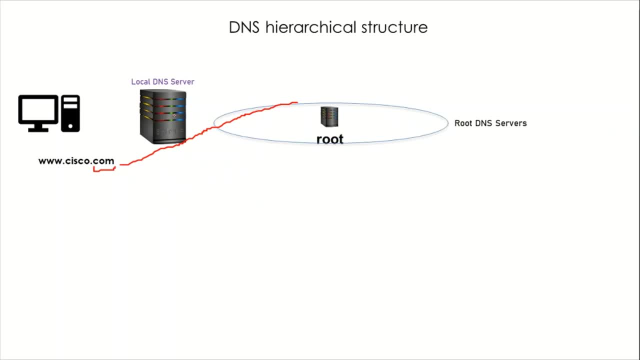 this root level will forward or will give an IP address to the local DNS server to get connected with the com part of the domain server, which we call a top level domain servers. So in this case this will give us an IP address for this server, com server.